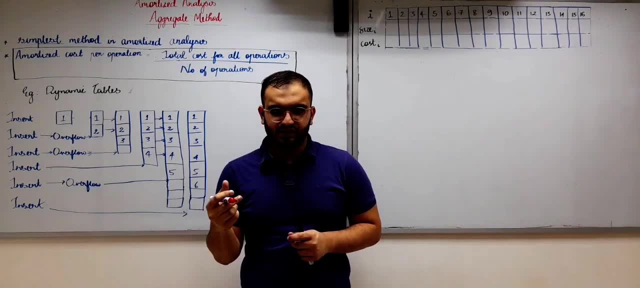 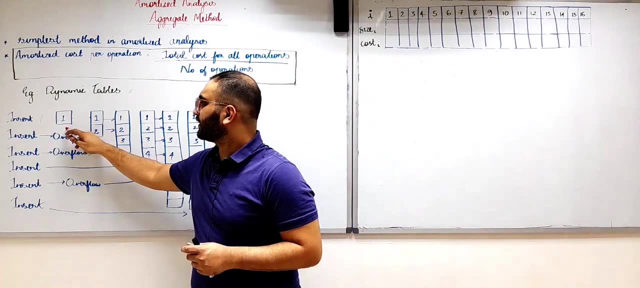 dynamic array in which, if we keep on inserting elements- okay, and suppose here this is the first insert, we have inserted the first element. okay, initial size of the dynamic table was zero, So we inserted the first element. now the size is one. 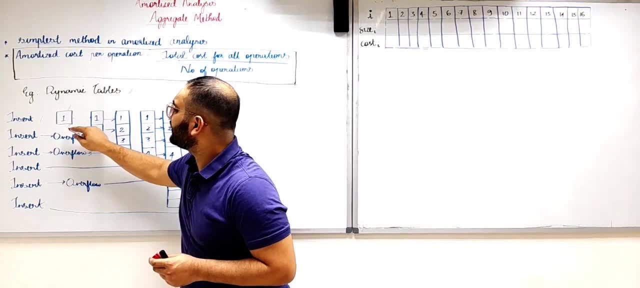 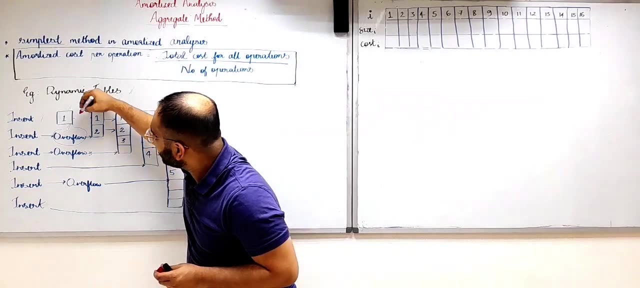 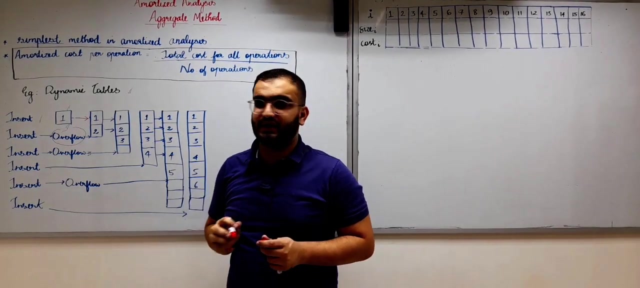 In the second insert. what happens is that now there is an overflow. the maximum size of the dynamic array was one. So now what we do is that we copy actually this element that was already in the array and we double the size of the dynamic array. 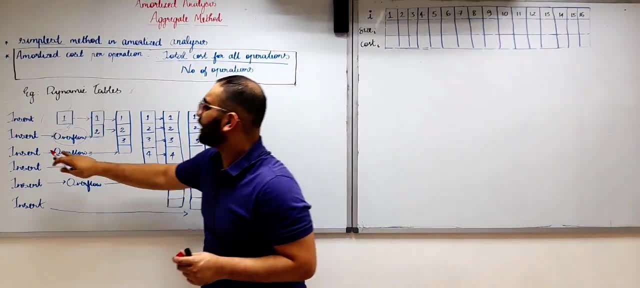 So now the size has increased from one to two. right Now we do the third insert in the, the third insert. again there is an overflow, that the size is two, but you are trying to include the third element. so in such a case, 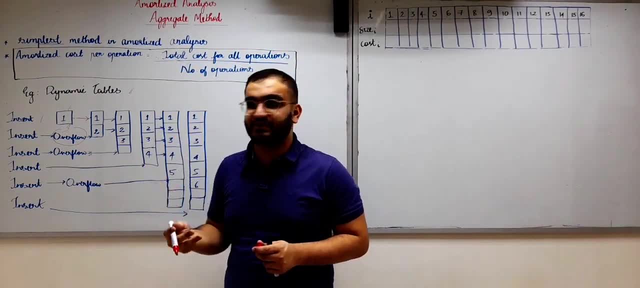 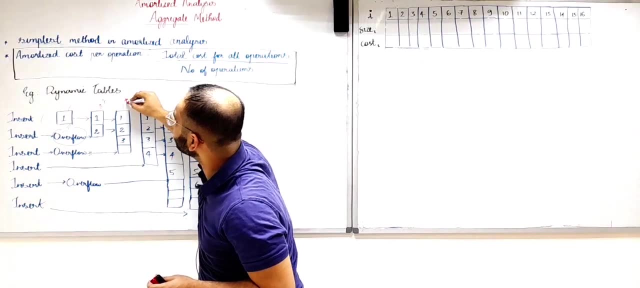 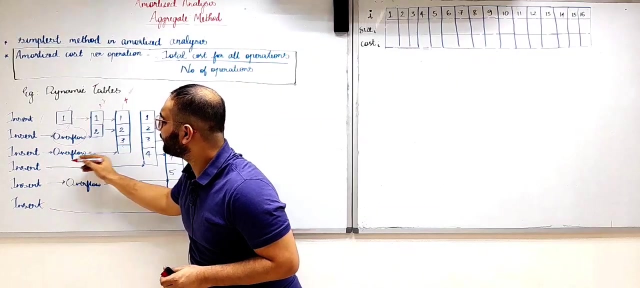 but you are trying to include the third element. So in such a case Again, the size doubles. from here The size was 2.. Now here the size becomes 4, right, And we insert the third element. So that is what we have done over here. In the case of the fourth insert- right, This fourth insert- there is no overflow because there is already a space left. 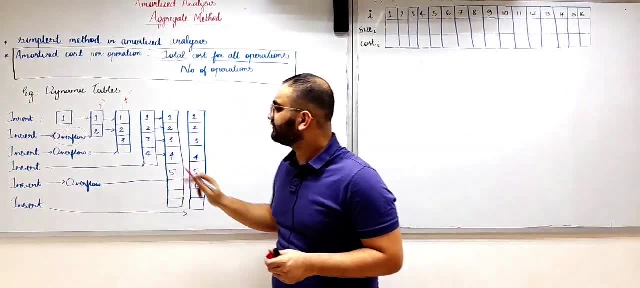 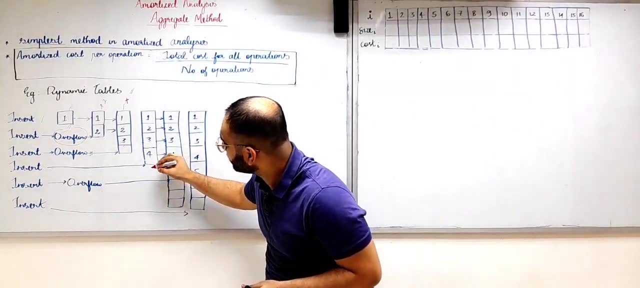 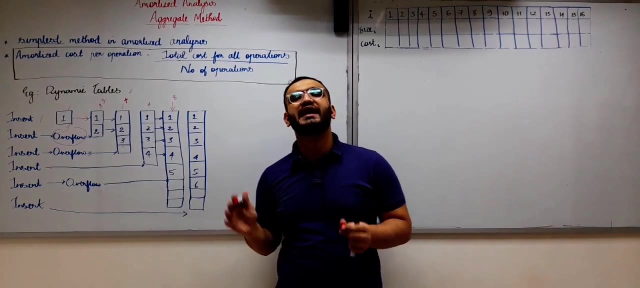 So we insert the fourth element. But when we want to insert the fifth element, there is again an overflow. So we double the size of the dynamic array And now the size is from 4.. From 4, the size has changed to 8. And we insert the fifth element. So this is how the dynamic table works. Every time there is an overflow, the size of the dynamic array will actually double, right. 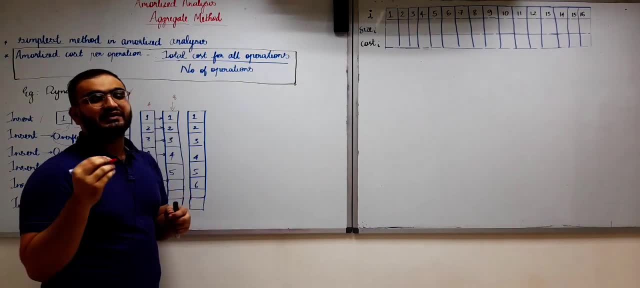 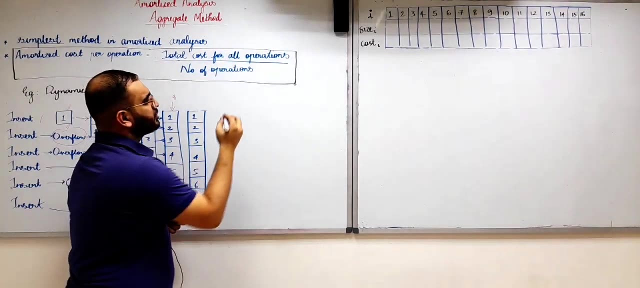 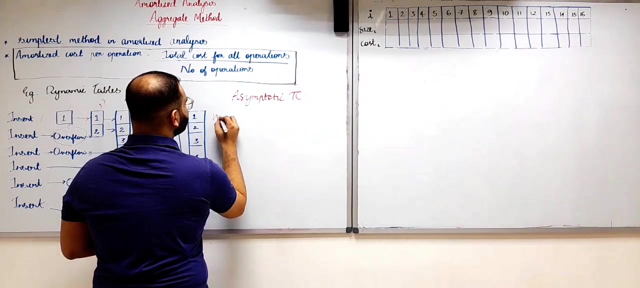 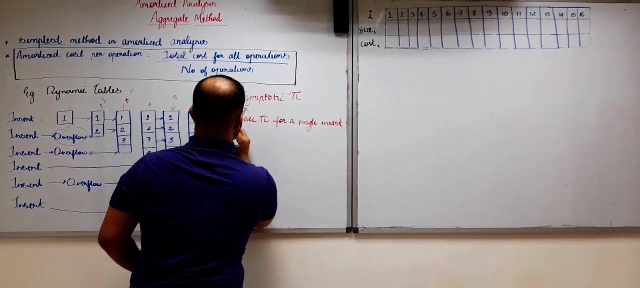 So now we need to actually find out the asymptotic time complexity. So now, if we find out the asymptotic time complexity, So now what is the worst case? time complexity for a single insert. right, This is what we need to find out. 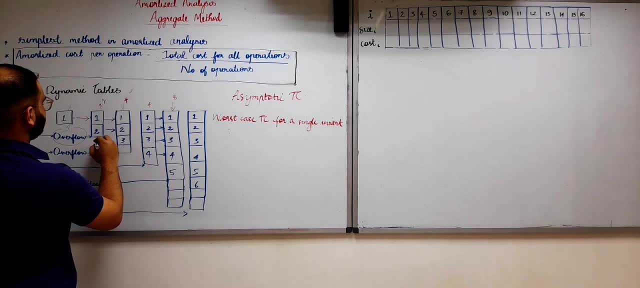 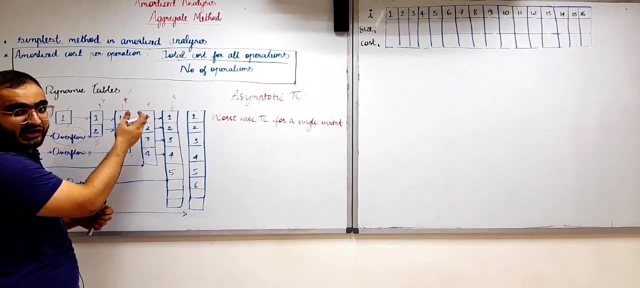 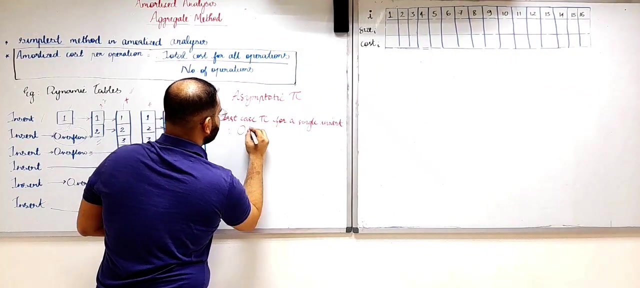 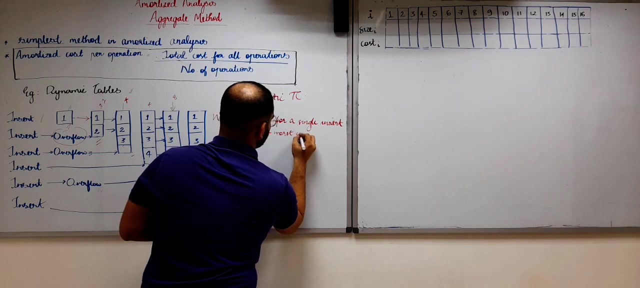 So for a single insert. as you can see, in all these cases- this case and this case, that for a single insert- what we had to do is that we had to copy the previous elements- All right, All those elements- and insert the new element. So the time complexity in such a case is order of n, right, Whenever there is an overflow, the time complexity is order of n. So this is my worst case which happens in case of overflow, right. 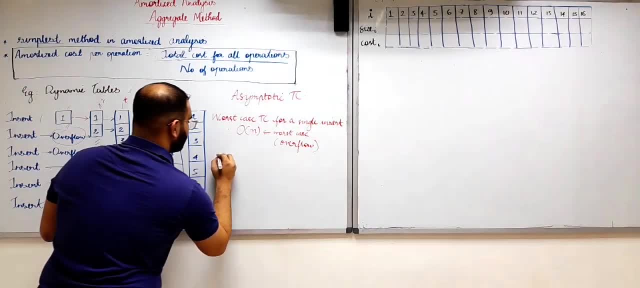 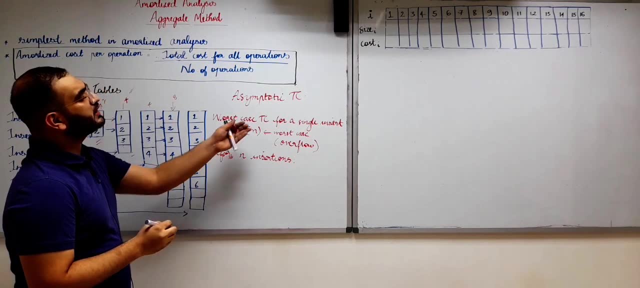 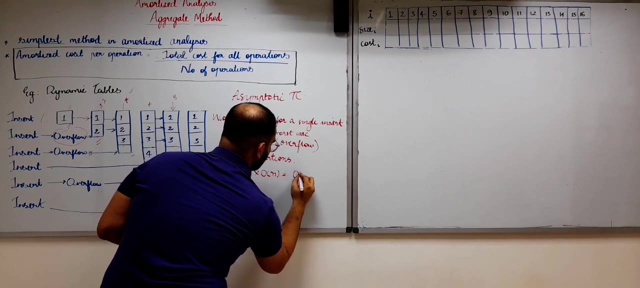 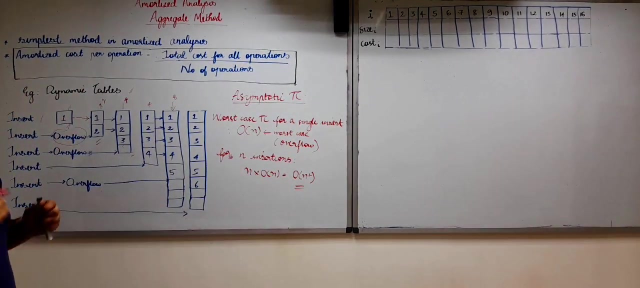 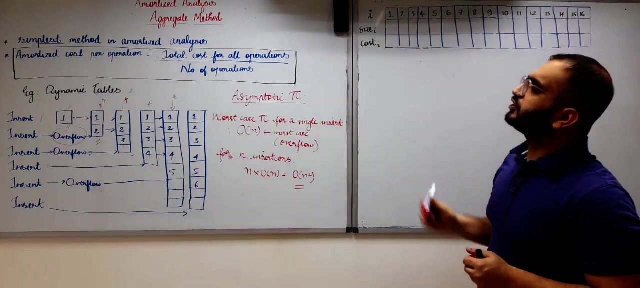 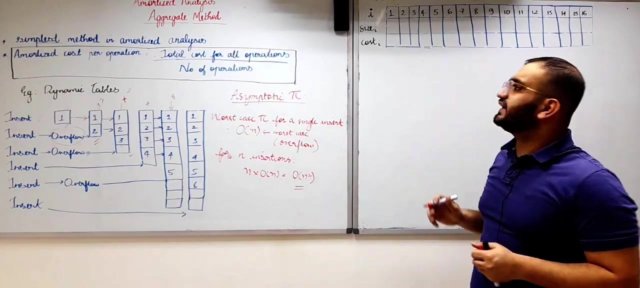 Now what is the worst case time? complexity for n insertions. So of course we will multiply the number of insertions into the worst case time complexity For a single insertion. we are going to have the ohm quantity of What we canunky do is. we are going to show how to use this in a flat table. 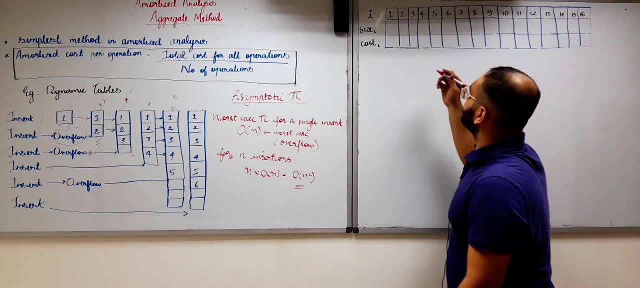 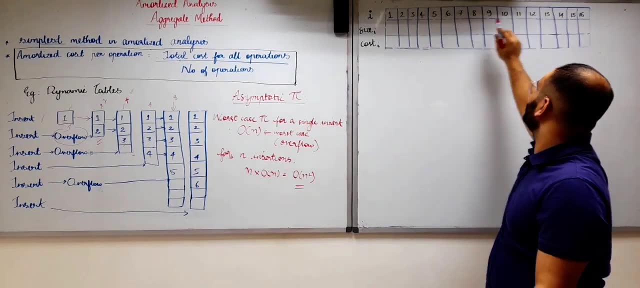 So here I have an acronym at the end. Here I have an acronym at the end of dynamic tables, right, so now this I over here denotes the number of insertion. like this is the first inch insertion. second insertion: it goes on up to the 16th insertion. size of the I denotes: 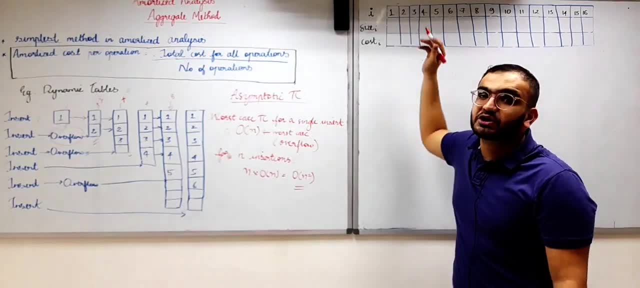 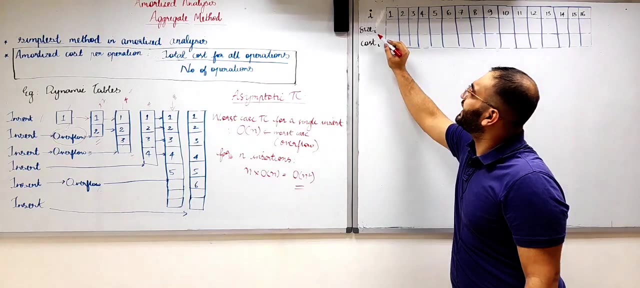 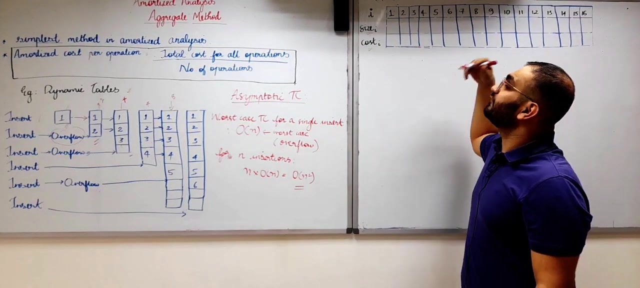 the size of the dynamic table at that particular I insertion, right? so when I say size of 4, that means what is the size of my dynamic table at the fourth insertion and cost of I over here denotes what will be the cost of the i insertion like. if I tell you, if I ask you, cost of seven, you will. 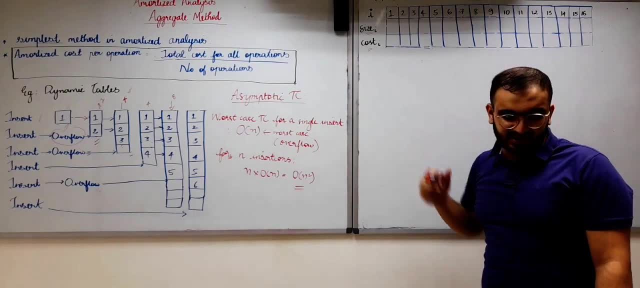 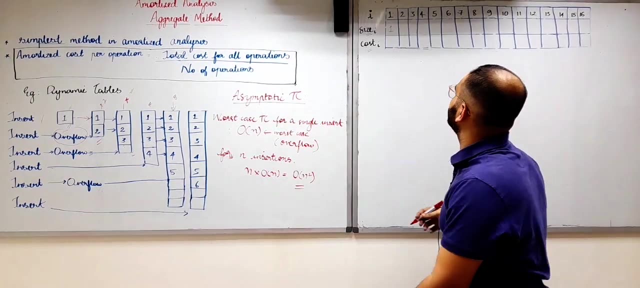 that will actually mean what is the cost of the seventh insertion. right? so now over here. if in the first insertion the size of the dynamic table is one, as you can already see over there, and in the second insertion the size of the dynamic table will be two, and in the third insertion 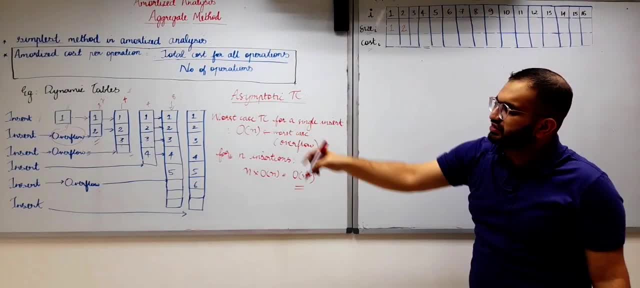 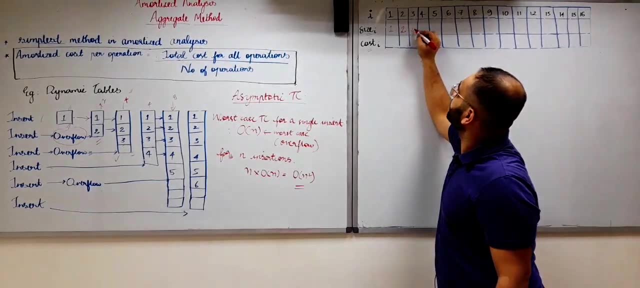 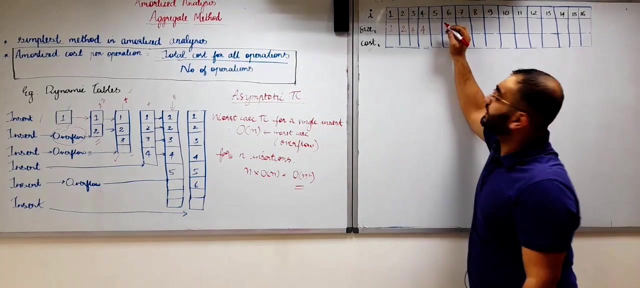 because here there will be an overflow, as I said, in this case over here. so that is why the size will actually double. it will not be three, it will double. so this will be four. in the fourth insertion: no overflow. the size will total. size of the dynamic array will remain same: four. but in the fifth, 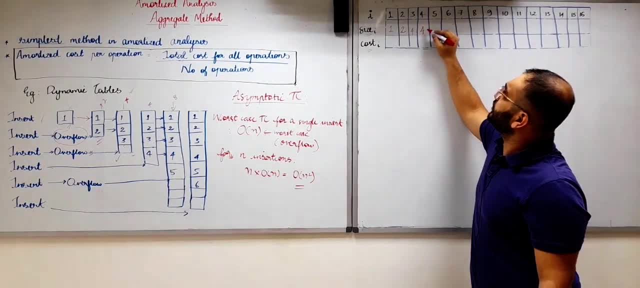 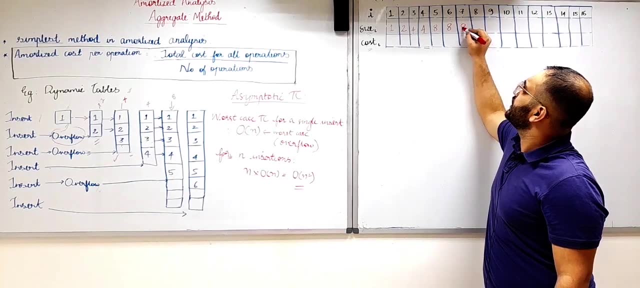 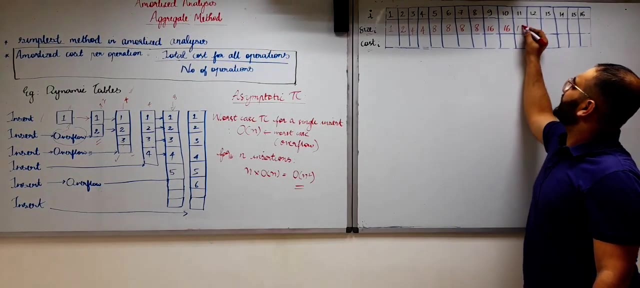 insertion the size of the dynamic table. because of the overflow, it will actually double from four to eight. in the sixth insertion, again there is no overflow, so I'll fill it now. eight. now, here again there is an overflow, the so the size will double from eight to sixteen. so again there are no. basically there are. 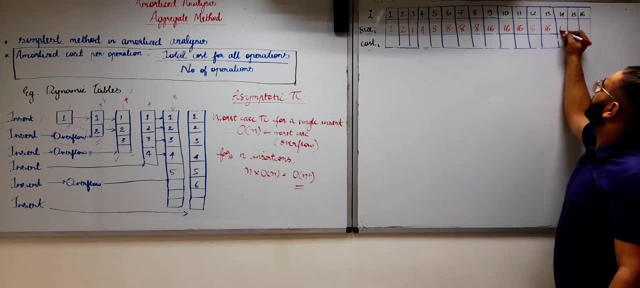 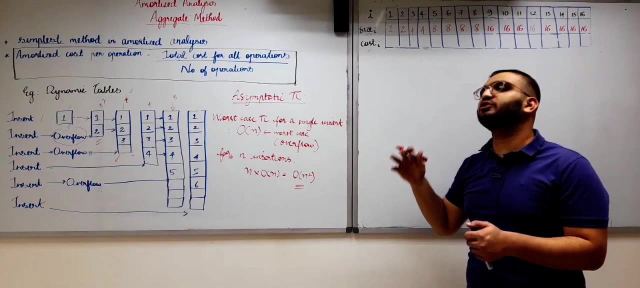 no overflows, so the size will remain same. so it will remain same over here. and in the case of 17 insertion, the size of the dynamic table would have been from 16 to 32. so now we have to find out the cost of each insertion, right, so for? 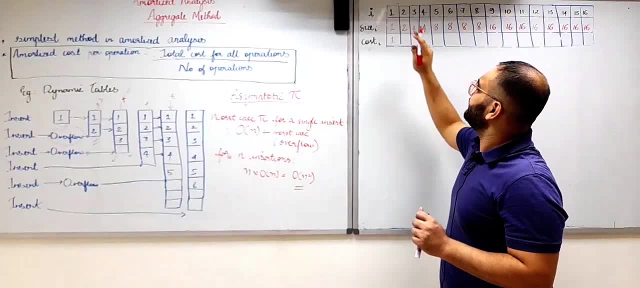 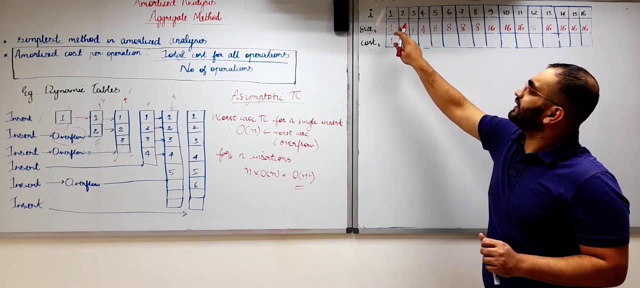 the first insertion, the cost will remain one, because only we are doing one insert. for the second insertion, the cost will actually become two. the reason is we are. the cost will actually become two. the reason is we are actually copying the first element that was already in the dynamic table and 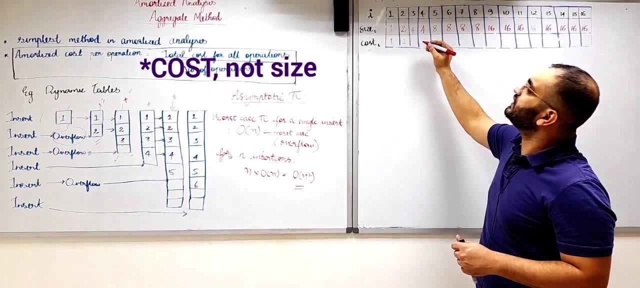 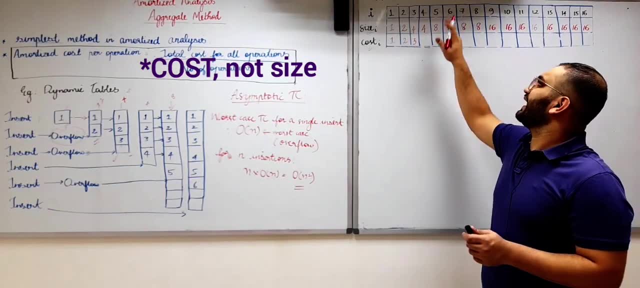 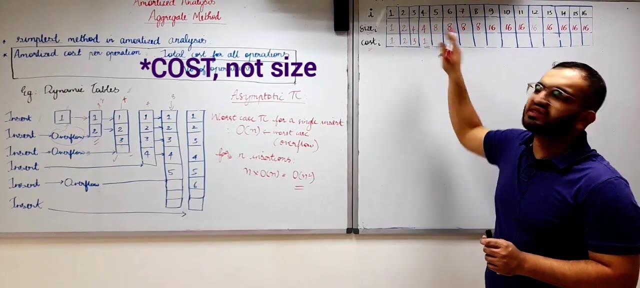 then inserting the new element, so the size becomes two. in the third insertion the size will actually be three. the reason is we are actually copying the first two elements and then inserting the new element, but in the fourth insertion the size will just be one because there is no overflow. we are just 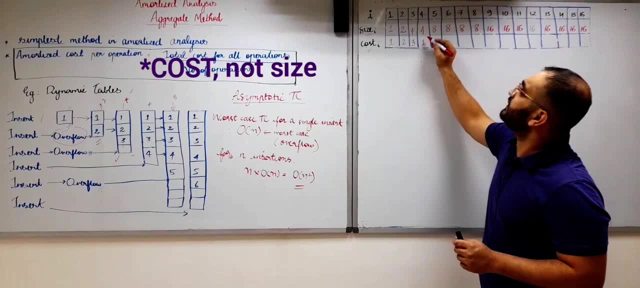 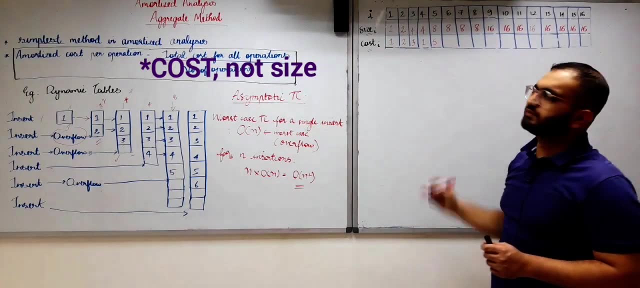 adding the new element. for the fifth insertion, the size will be the previous elements that are in the dynamic tables. until now, four elements are there, plus the new element that we are inserting, so the size will be five. for the sixth element, the size will be actually one, because there is no. 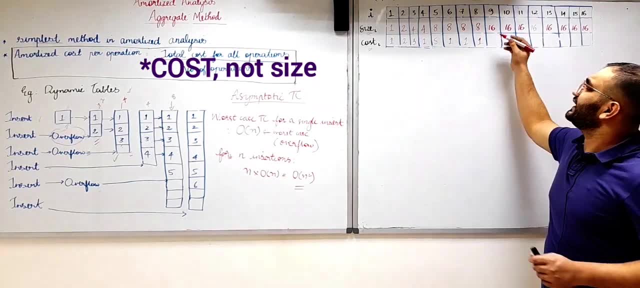 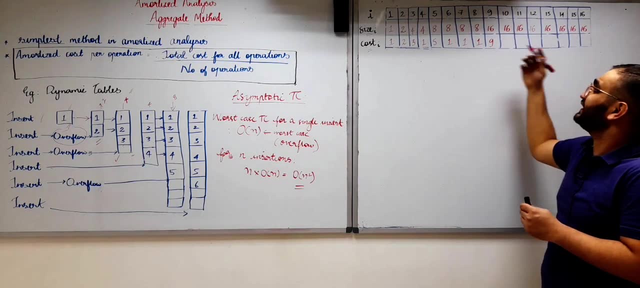 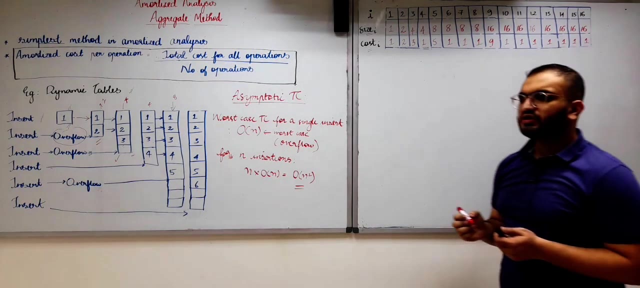 overflow. seventh, also same. eight, also same, but for the eighth element the size will be actually nine, because the eight previous elements and this new element. so eight plus one, nine, this will be one, one one. so all of these will be one. so now if we actually want to summarize this table, 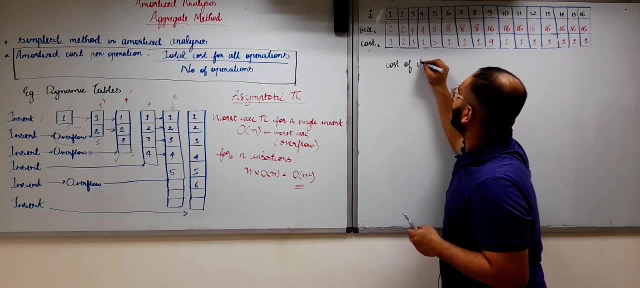 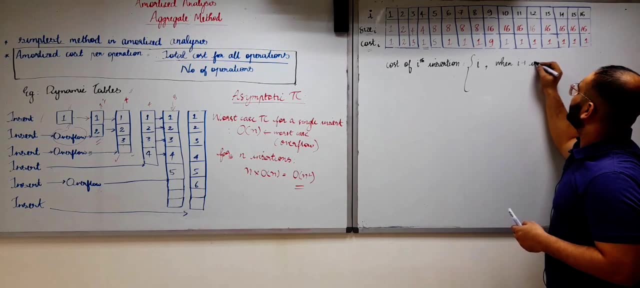 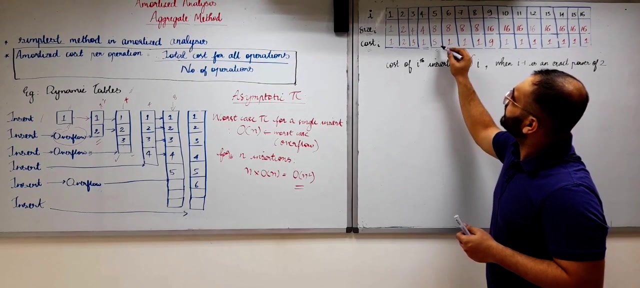 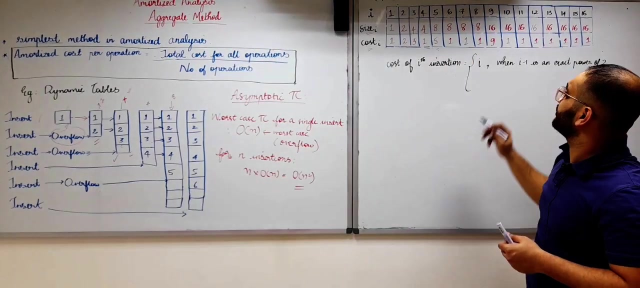 we can write. it is in this way: cost of ith insertion is equal to I. when I minus one is an exact power of two. okay, so you can identify over here. actually, the of I over here is five. so when I minus one, four is exact power of two in this case. 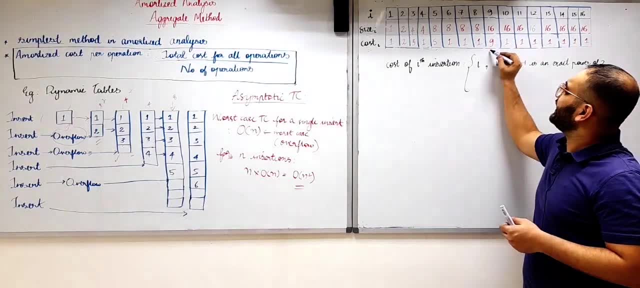 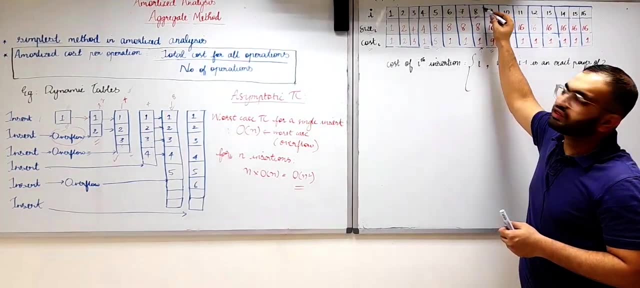 in the same way. here we are getting the cost as I. that is nine itself. cost of I is equal to I, and again you can see over here, the I minus one or eight is an exact power of two. so this is how we summarize this table, or else: 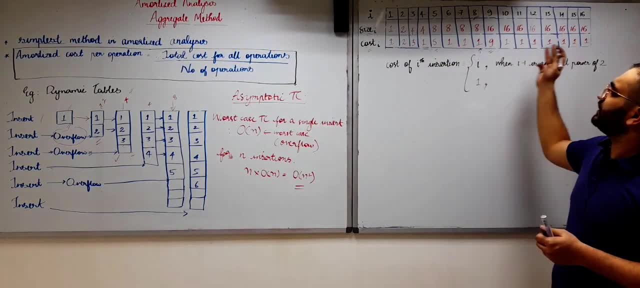 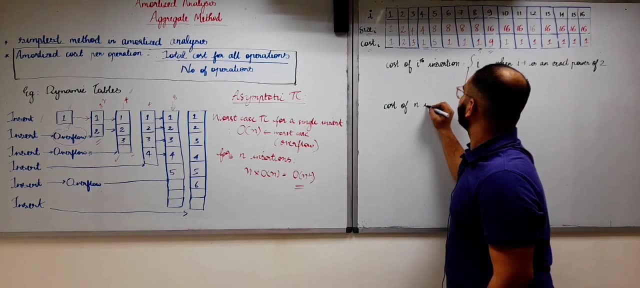 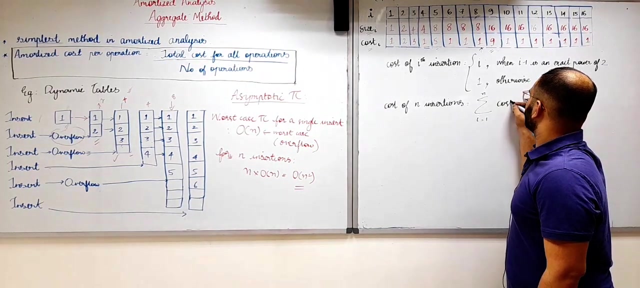 the cost will be one, or else you can see in the rest of the places the cost is one otherwise. so now, if we want to find out the cost of n insertions, we will do a summation of I is equal to one to n cost of I, right? so this is basically. this is. 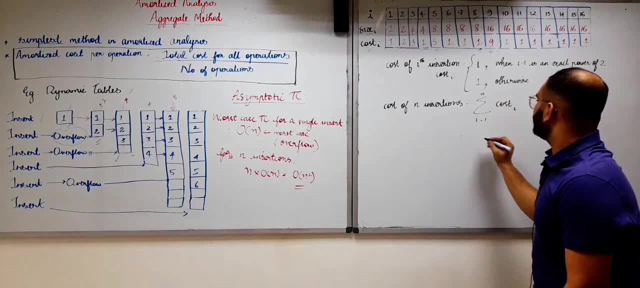 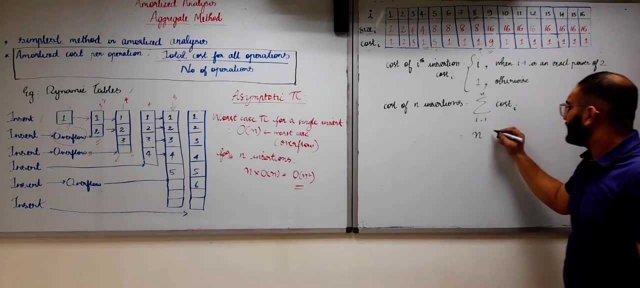 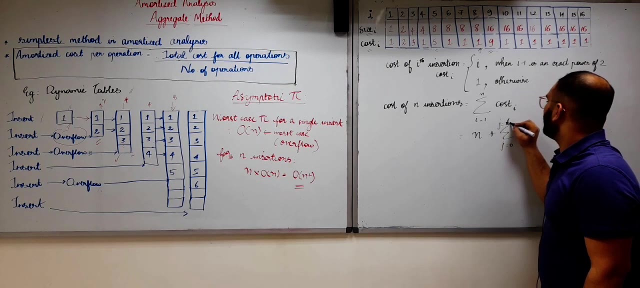 the same thing. cost of I. so over here this will be n, because we are considering that every insertion is taking one, one unit of time for the time being, plus summation of J is equal to zero to J is equal to log of n minus one. I want you to tell me in the comments that why I am taking J zero as the lower. 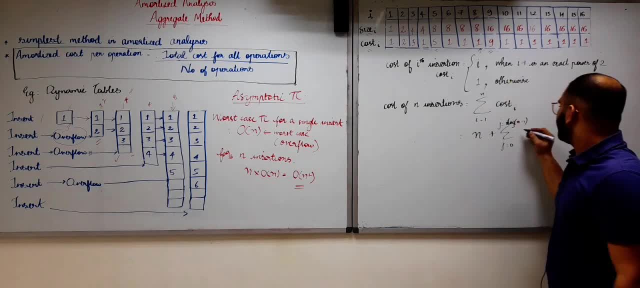 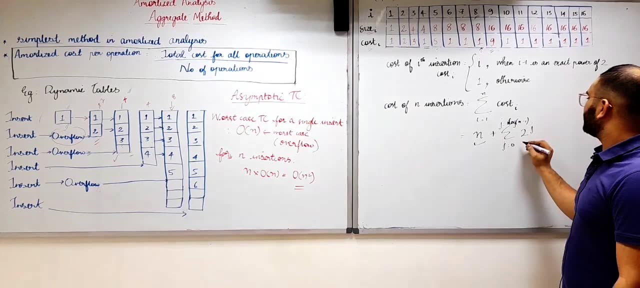 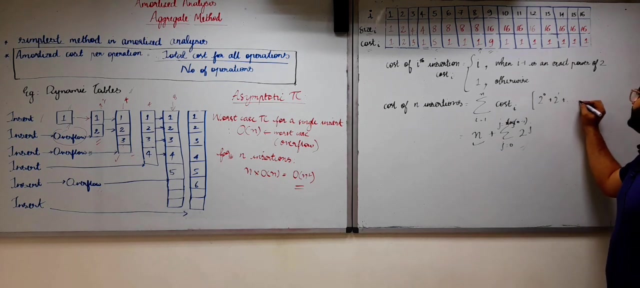 bound and n log of n minus one as the upper bound, and this will be two of J. so if you look at this series, this is already n. but if you look at this series, it will be something like this: from two of zero plus two of one up till two of. 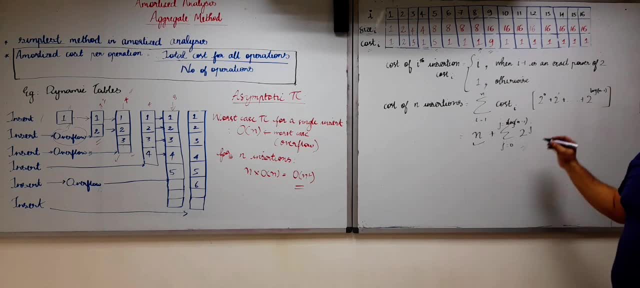 log of n minus one. so the sum of this series is basically, as you might already have learned, the sum of the series is calculated in this way: into R of n minus one divided by R minus one. in this case, a is two. raise to zero or one. 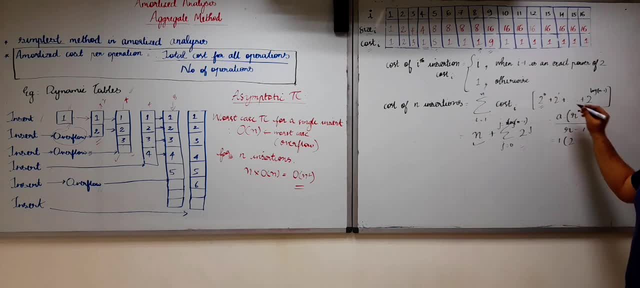 and R is two and n. the total number of elements is log of n minus one plus one element. so log of n minus one plus one element minus one, divided by, as we over here, R is two, so over here the denominator will be one. so this is again. 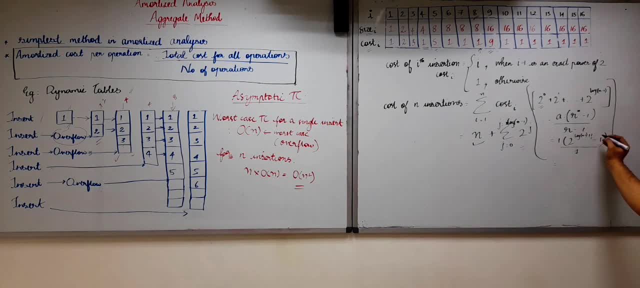 a rough calculation that I am doing. we can write this one over here as log of two or two by two. so this will be log of n minus two plus one. so the following thing from a common include a limit not going to quantity 1 plus log of 2 by 2.. So this will finally be. this is finally going to be as log of. 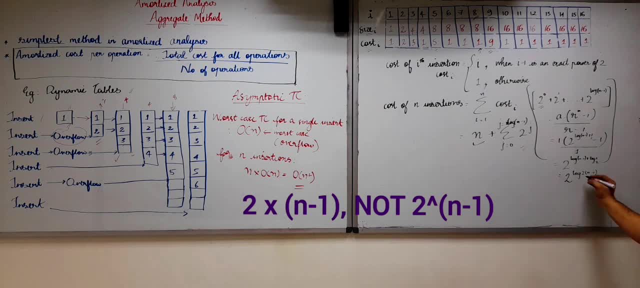 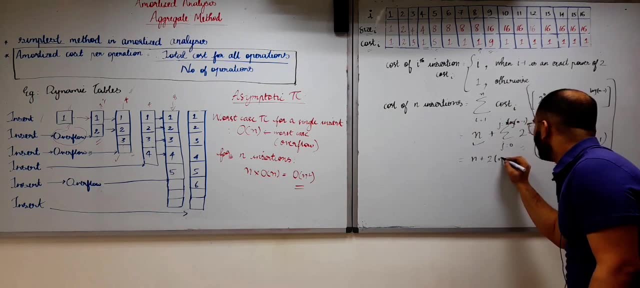 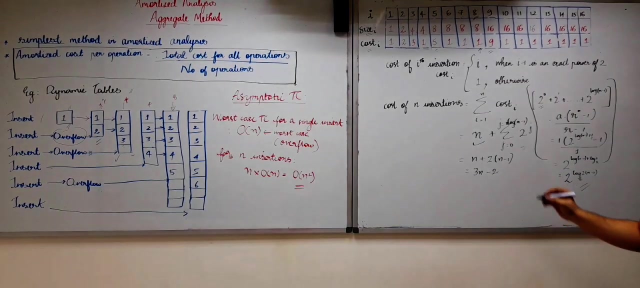 2 raised to n minus 1, right logarithmic properties, This summation will finally come out as n plus 2 into n minus 1.. So this is something 3n minus 2, right. So this is less. 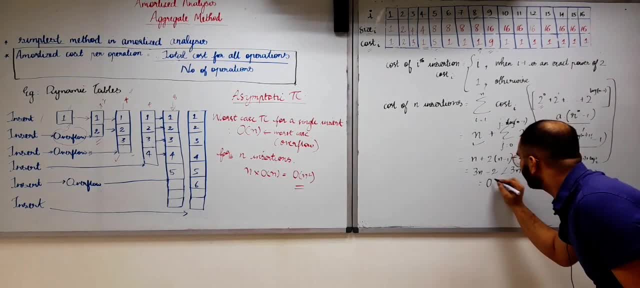 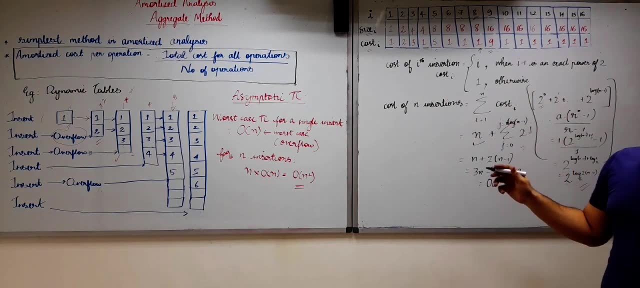 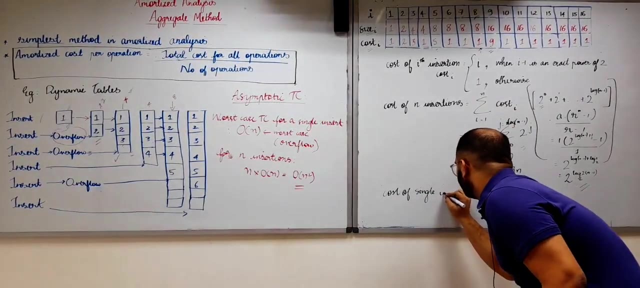 than 3n, or you can also call it as order of n. So this is the cost of n insertions in a dynamic table, if we find it out with the help of aggregate method, and also to find out the cost of single insertion with the help of aggregate method, with the help of that formula. So the total cost 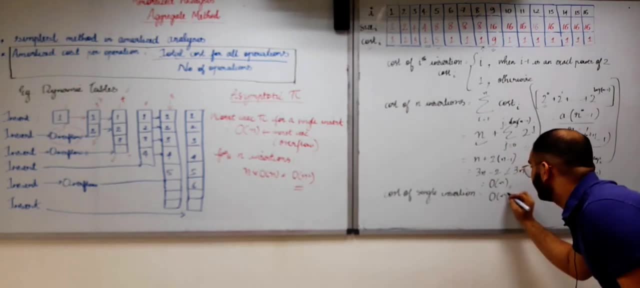 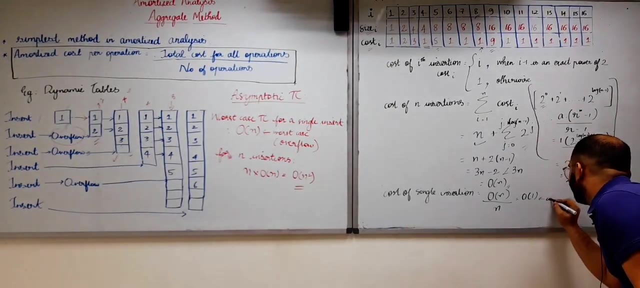 for n insertions is order of n divided by the number of insertions is n. divided by the number of insertions is n. divided by the number of insertions is n. So the total cost is order of 1 or constant. So I request you to actually keep in mind this.